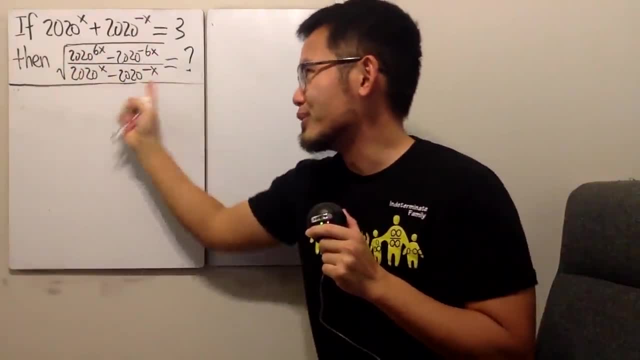 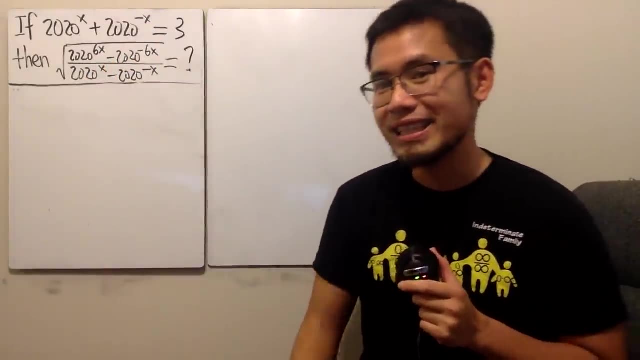 solve x right here, because we're trying to compute this expression. If you solve for x right here and I plug in the x into 0 here, that's not going to be really nice. But anyway, as always, please pause the video and try this first. 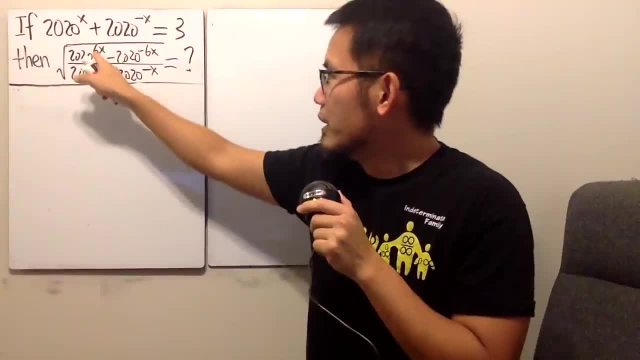 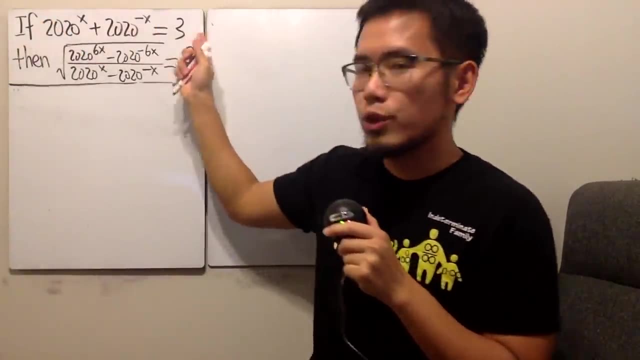 Alright, hopefully it gets a chance to try it. Here we see we have the 6x power and this is negative 6x power. It seems like we should just go back to the original equation and raise both sides to a 6 power. huh, No, don't do that. 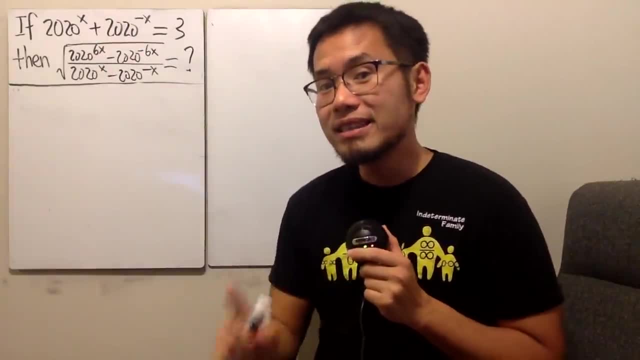 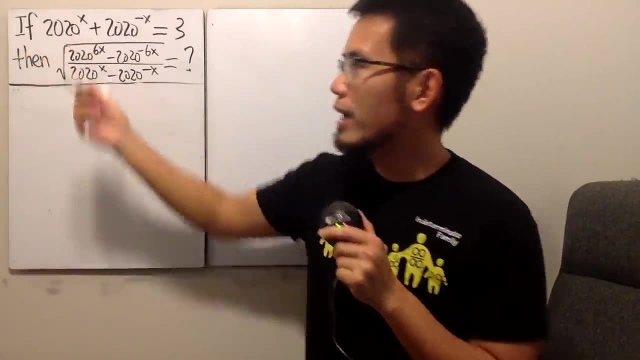 neither. That's going to be pretty bad on the left hand side. Instead, though, this right here actually can be factored in, and we are going to do that. By the way, I do not want to write down 2020 to the x power so many times, So let's do. 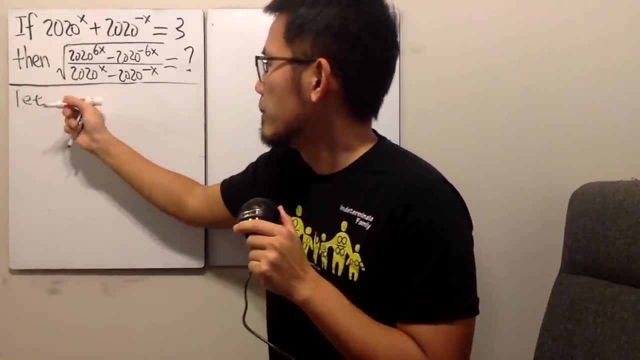 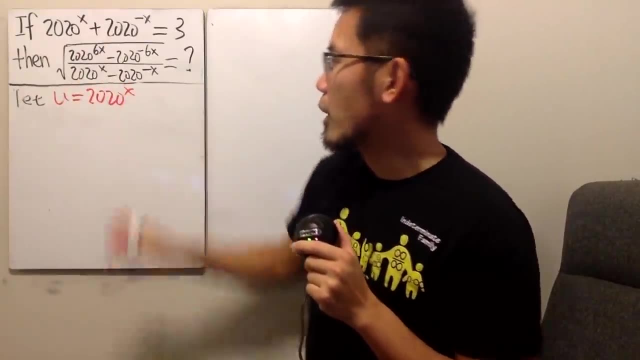 the following: I'm just going to do a substitution. I will select a variable- let's say u, because I like u, and I will be calling this to be 2020- to the x power. So the original equation becomes u plus u to the negative 1, that's equal to. 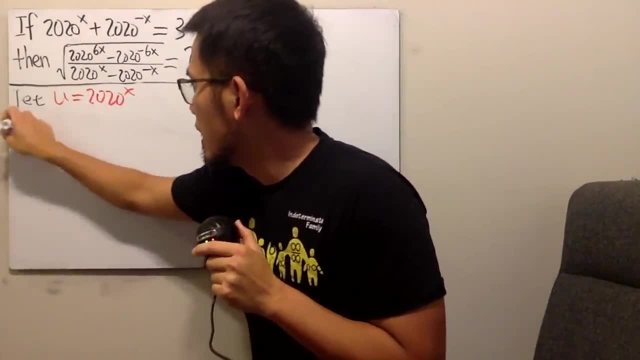 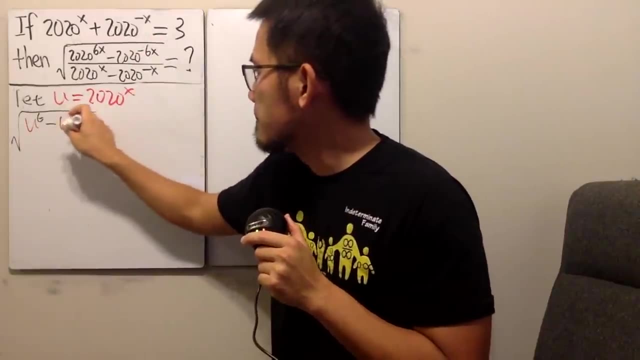 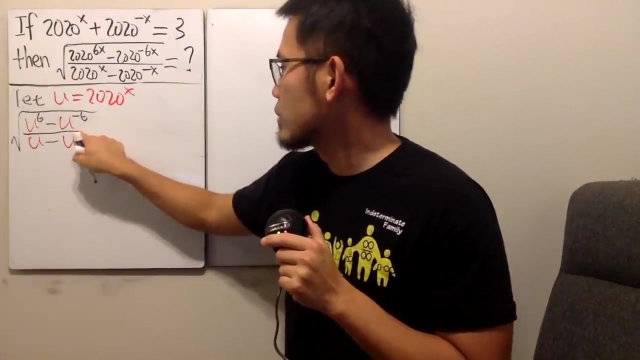 3. And this expression is going to be the square root. and here we have just u to the 6 power, Minus u to the negative 6 power over u, and then minus u to the negative 1 power, like this, and that's how we have to compute, Alright? so now let's see what. 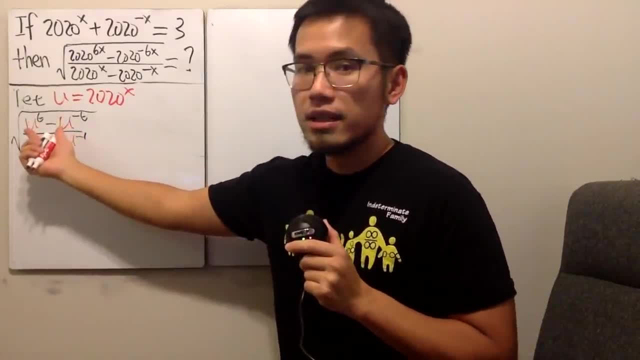 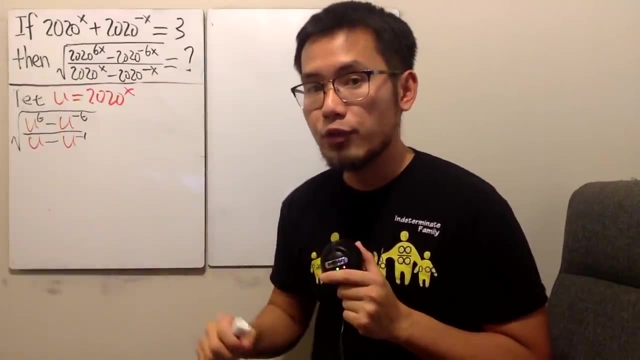 we can do with this. Have a look. This right here is the difference of 2 to 6 powers, So we can look at this as the difference of 2 squares or the difference of 2 cubes. It's easier to look at this as the difference of 2 square first, and 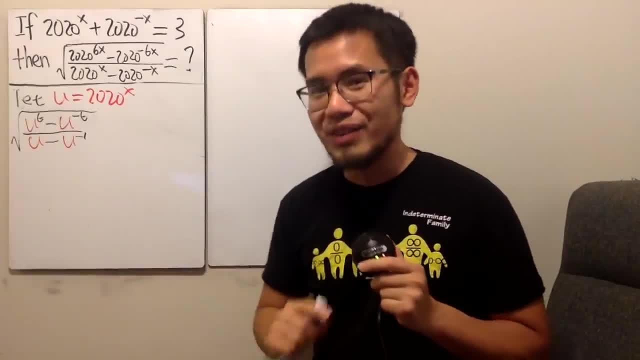 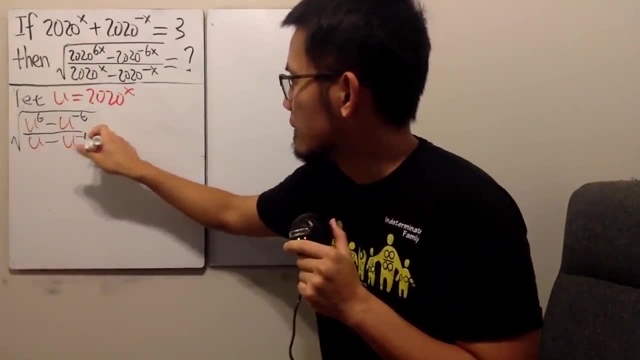 then we factor it If you want to do it the other way. in fact, I have a video on that already. It's kind of tricky, so check that out if you would like. Anyway, here we are going to look at this as the following: We will just break this down. So: difference of 2 squares. 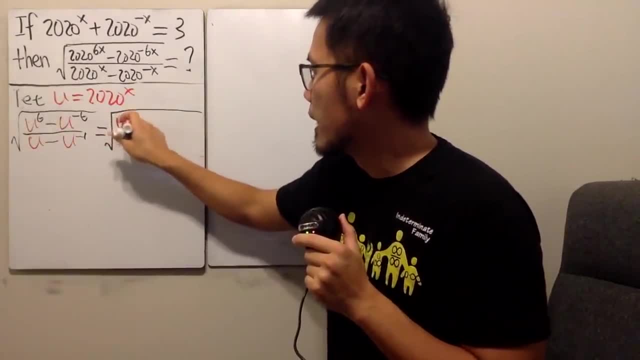 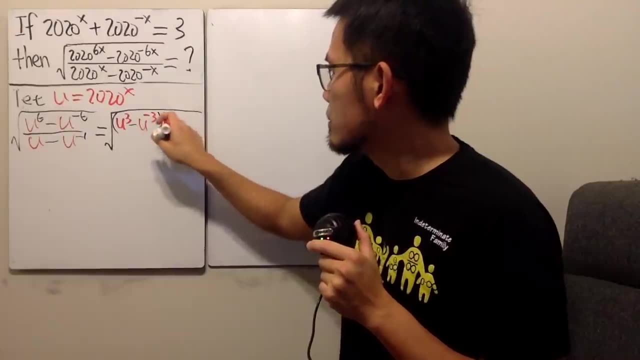 So that means the first term is u to the third power, and then we will have to minus u to the negative third power, like this. and then we have another one which is u to the third power plus u to the negative third power, like this: Alright, and then this is divided by that denominator which. 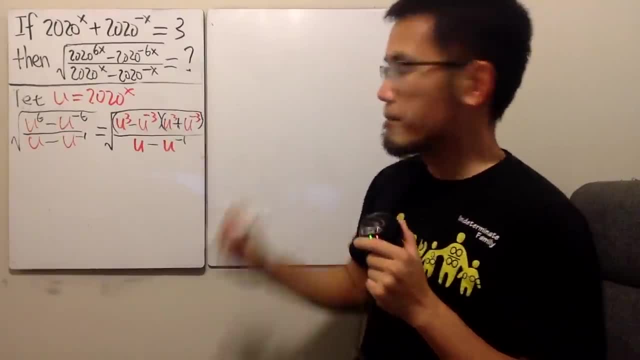 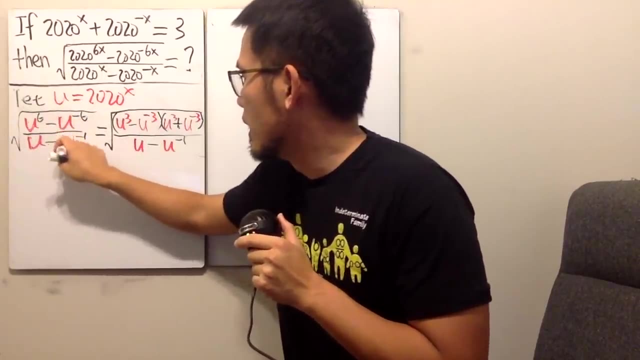 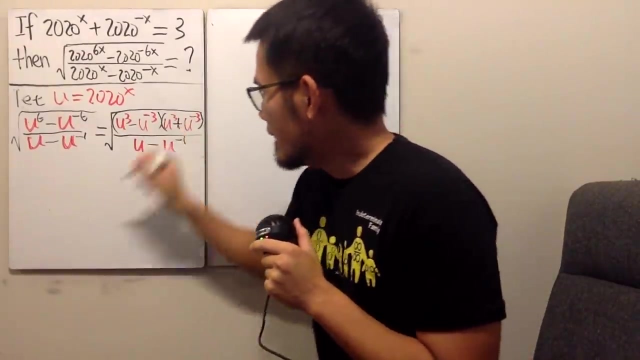 is u minus u to the negative 1.. Pretty good so far, and let me make the? u more visible for you guys. Better, Alright, now. what can we do next? We'll just keep factoring and hope for the best right. So right here. let's see if I can fit in everything right here. In fact, this is not the 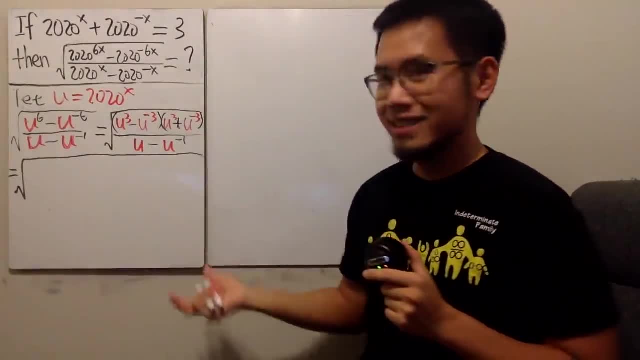 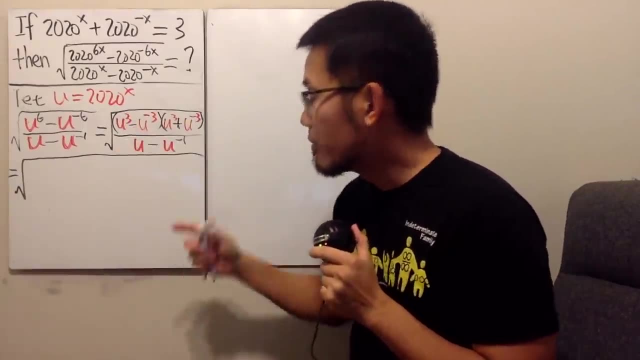 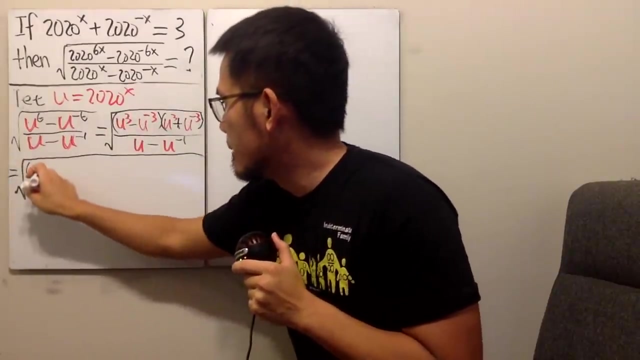 first time I'm recording this, because the previous times I failed on fitting everything onto the board. so life as a youtuber with small boards. Anyway, this right here factoring as the difference of two cubes, The first factor is going to be u to the first power, and then minus u to the 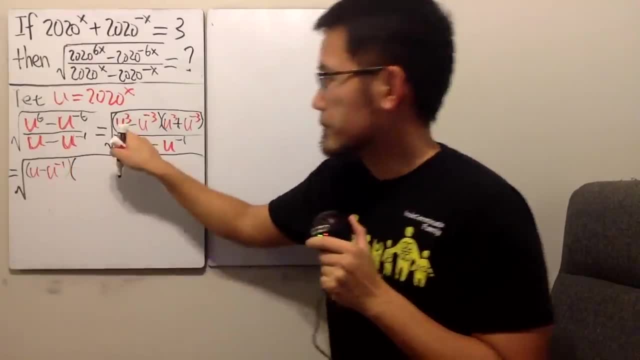 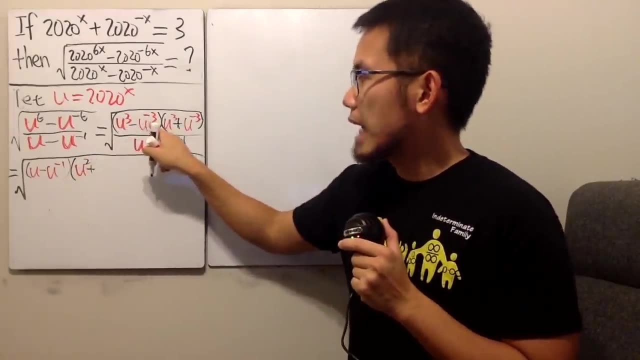 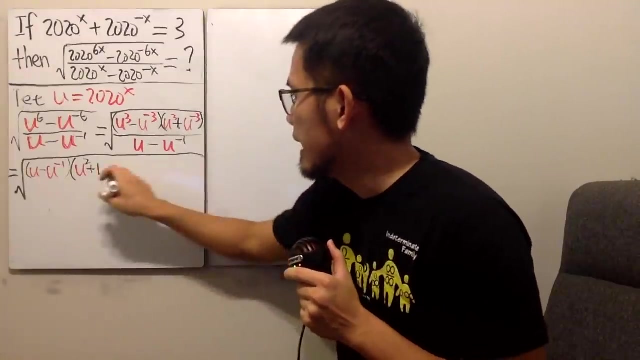 negative one power, and then we will have to do the following: This is going to be u square, and then times that u to the third power, times u to the negative third power is just equal to one, so we have to add one to it. and then, in the end, we have to add the? u to the negative one power- square. 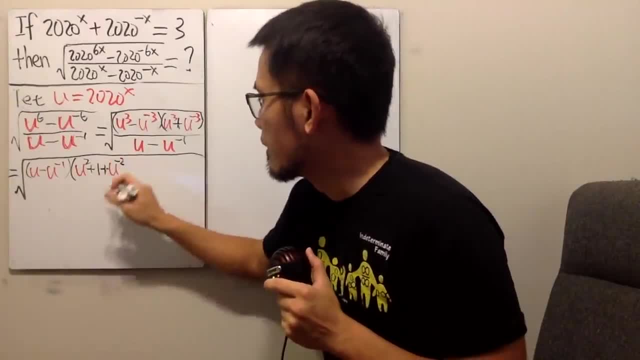 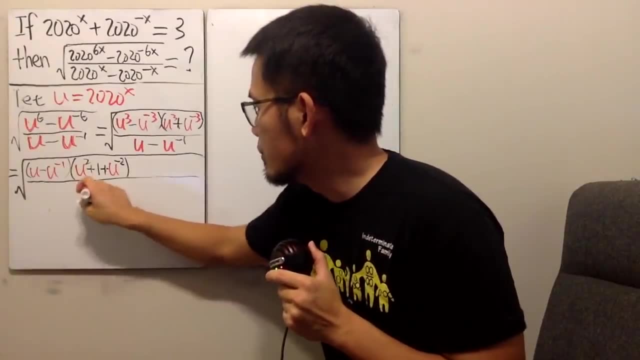 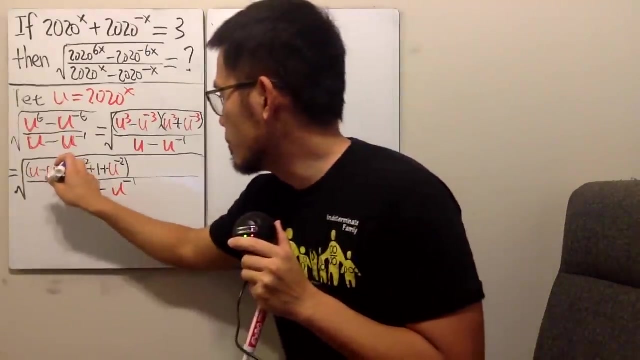 which becomes u to the negative two. so that's what we have, and this is actually pretty good, because on the bottom we really have this: which is u minus u to the negative one. yes, this is wonderful, because we can use the blue marker to cancel this out. all right, so now i just have to. 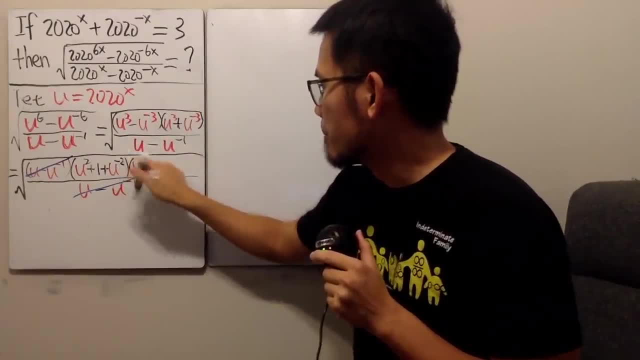 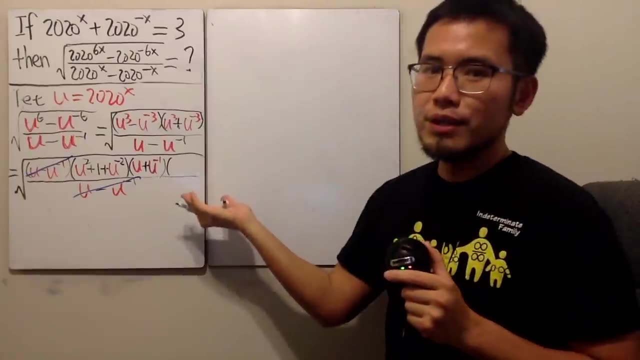 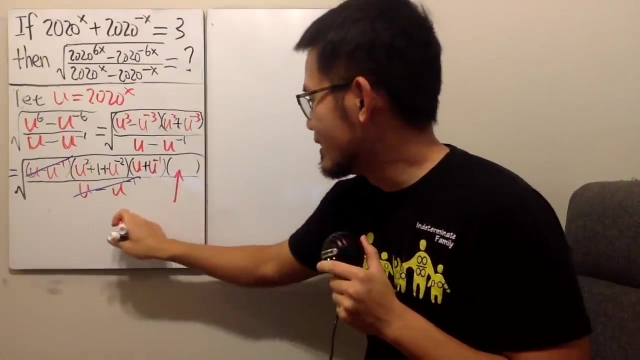 factor this right here, which will end up with u plus u to the negative one, and that's what we have. and then right here, see again, i failed it again, so i will try this. i will just indicate with the arrow: factoring this right here, we will end up with u, square, and then we have to subtract. 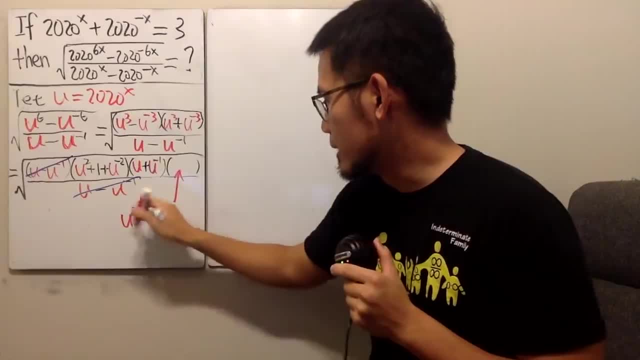 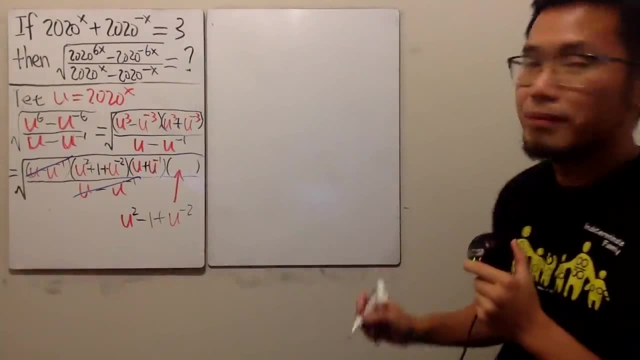 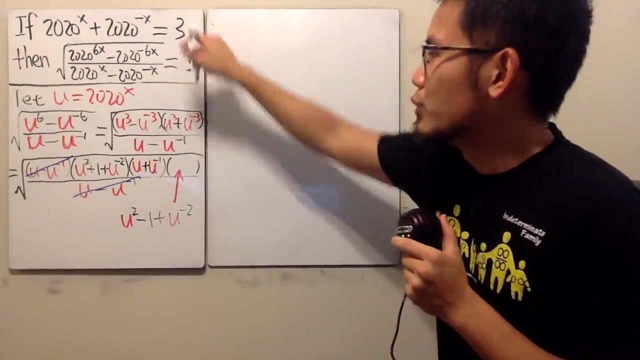 this times that, which is just one, which is similar to that, and then just add u to the negative two, so this goes here. all right, that should be okay. now let's see what else we can do. we do know this, though. this right here is our street right here, so that's good. 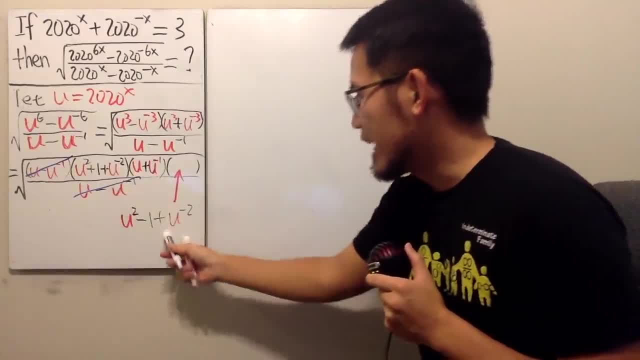 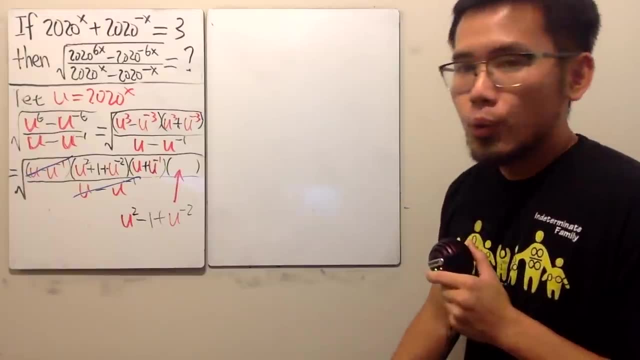 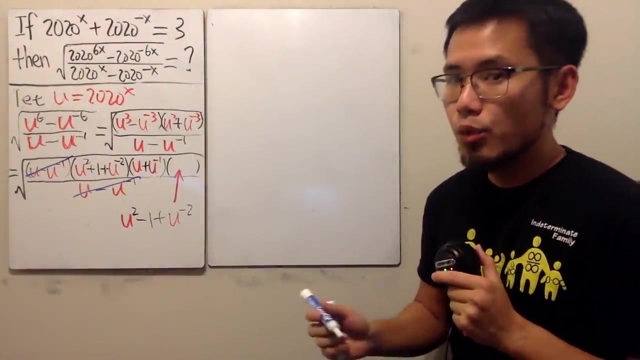 and, uh, the problem is that, what should we do with this? and that, uh, how to utilize this idea. well, the good thing is that things can happen with the blue marker. this right here can actually be factored in more, and the better thing is we can squeeze out this to help us out. so check this out. 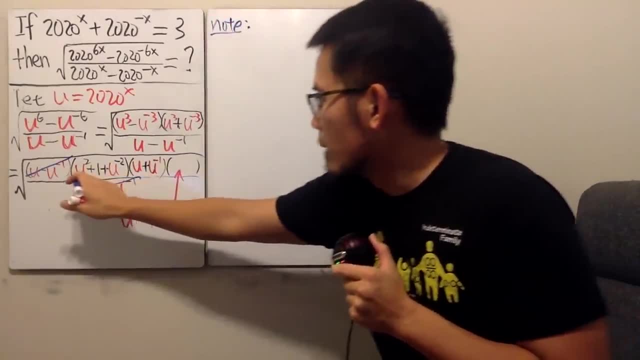 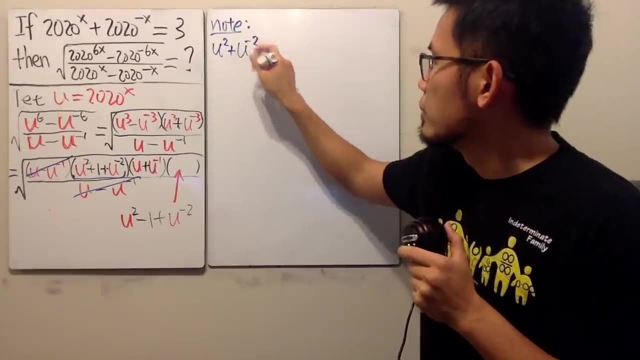 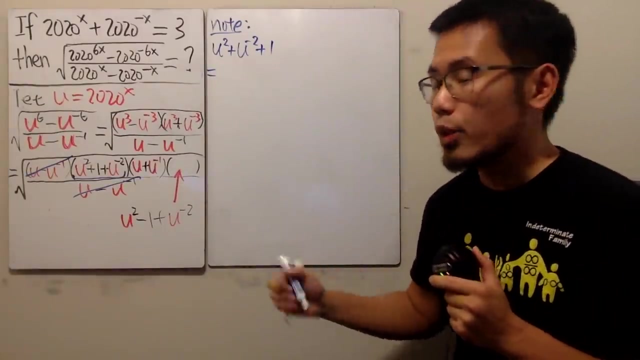 note right here, so i'll just put this down in blue for you guys. when we have u square plus, let me write this down first, which is u to the negative 2 and then plus 1. this right here is actually the same as a perfect square right here, and then we can actually complete a square with the first two terms. 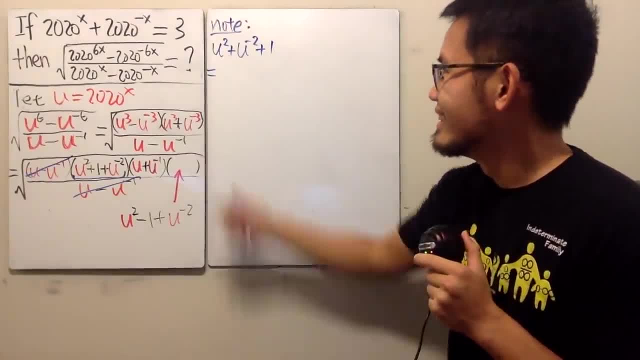 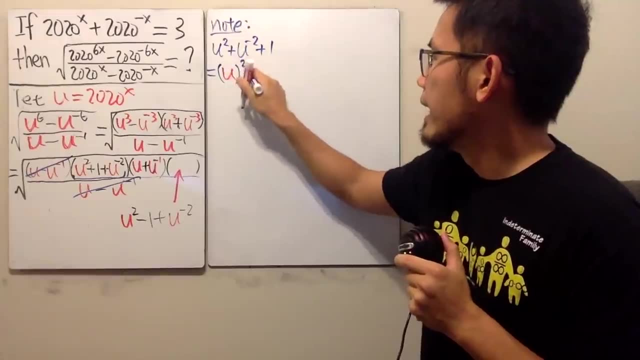 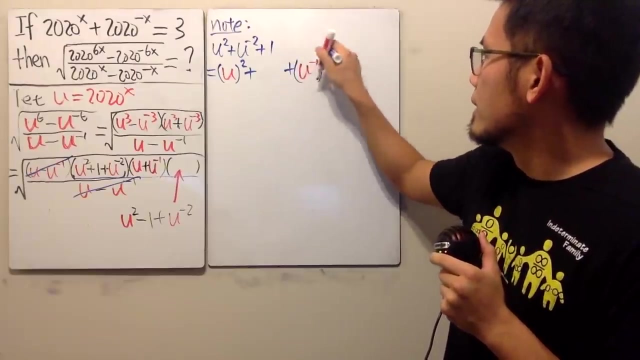 because it does look like a perfect square almost here. this is how we do it right here. you see, this is the same, saying u square and then plus something, and then let me just leave a space. plus this right here is the same as u to the negative one square, right, if you want to get. 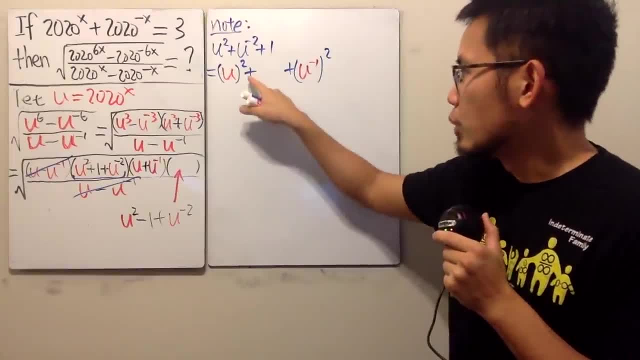 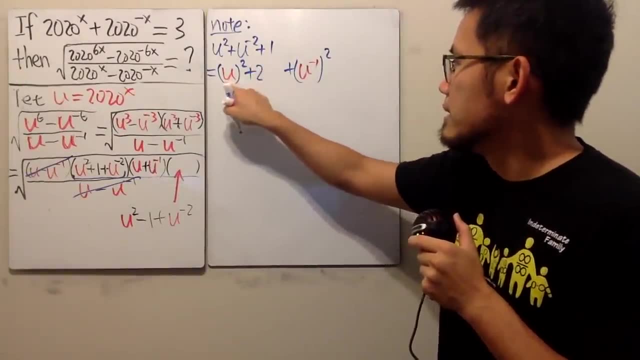 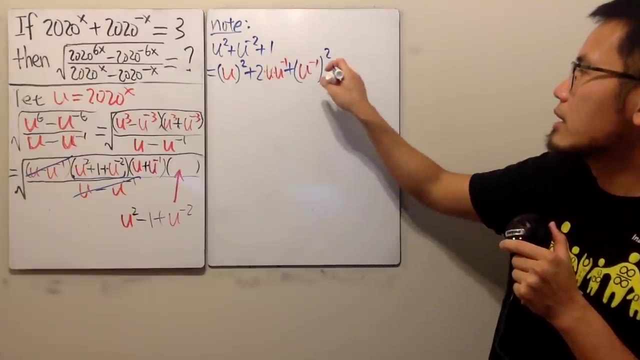 a perfect square right here, with the plus in the middle, and the reason i want to plus is because i want the plus right here in the middle. i will have to have 2 times this and that, namely u times u to the negative one, and then, don't forget, we still have the plus one after that. but you see this. 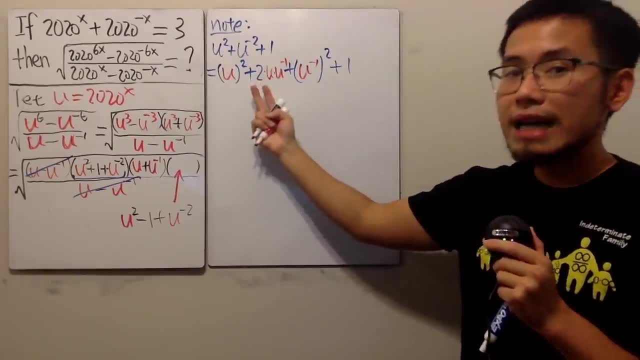 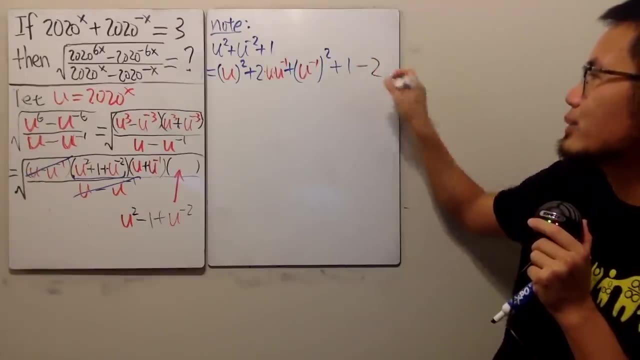 right here is actually just a two. so in fact, from here to here we're just adding a two right here to complete the square. but you cannot just add two of course. you have to just come back here and then minus two so that this and that can king. so when you don't measure the one, here you are actually. going to end up with something like this. so, once again, you will always have one plus one here and then, if you're able to put your square, so if you're able to kind of beside the square and you want to imitate the 21-1 square this time, these are just two 투 from the invisible one. okay, so now you know how to. चậy450. Musik. 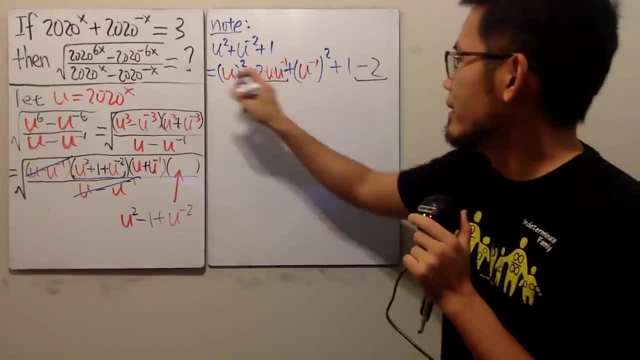 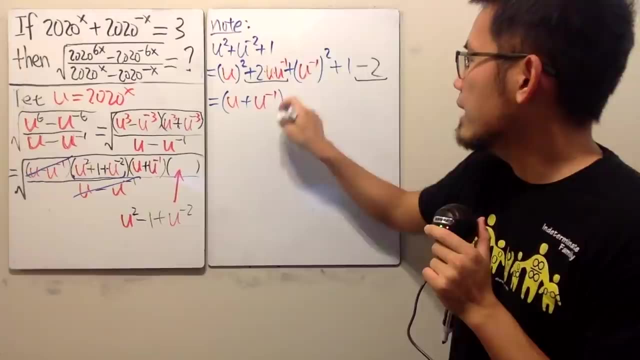 Cancel each other out, right, And we start being done. These three terms will just give us u plus u to the negative 1, and then raised to the second power, And, of course, 1 minus 2, we end up with minus 1.. 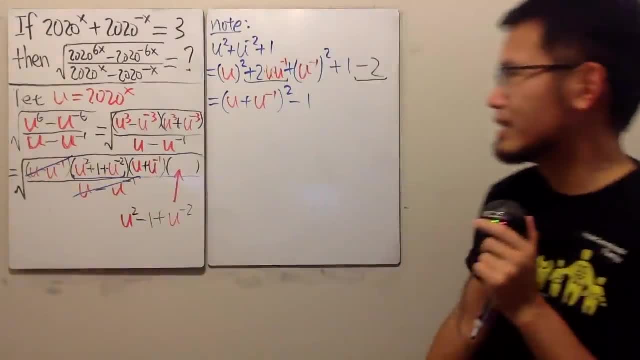 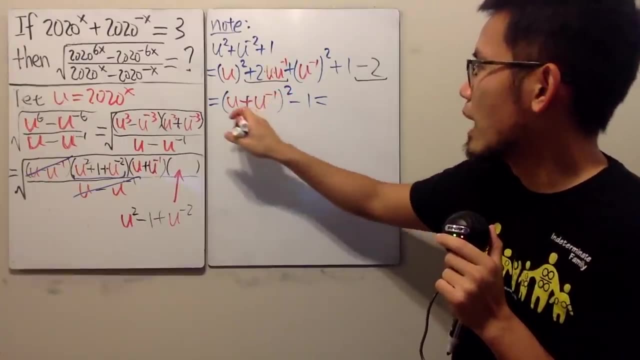 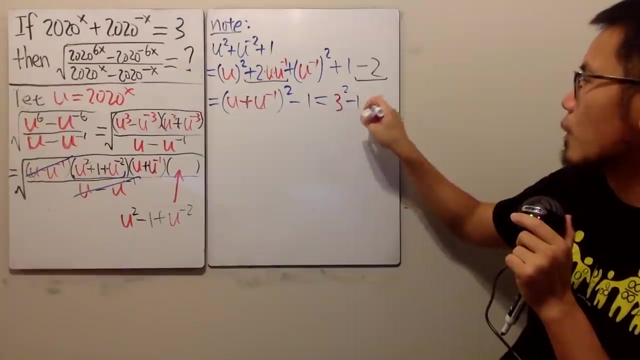 So this right here is going to be going for that Better yet. do we know the values? Yes, we do So. u plus u to the negative 1, this is nicely equal to our 3 right here. So this is 3 squared minus 1, and work that out, you get 8.. 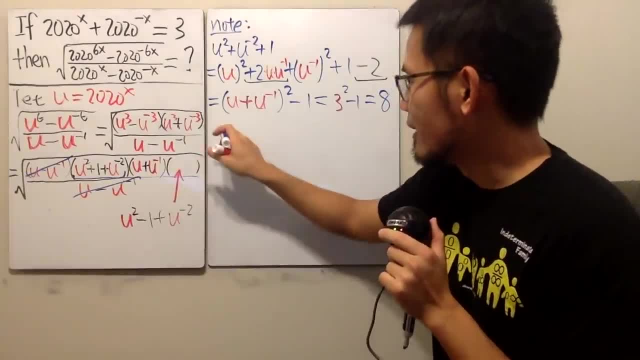 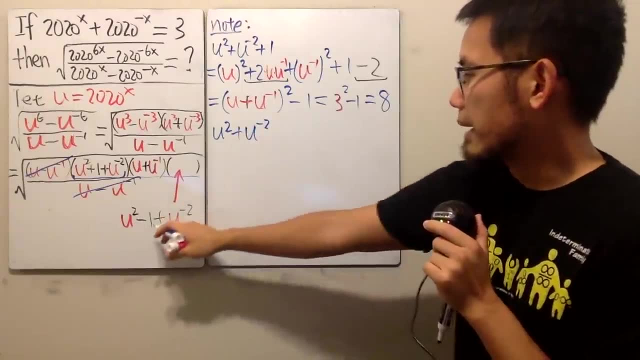 Great. Similarly for this factor here, if you look at u squared, and then again plus huh, that's really nice. plus u to the negative 2, but here we have minus 1.. Well, what do we do? 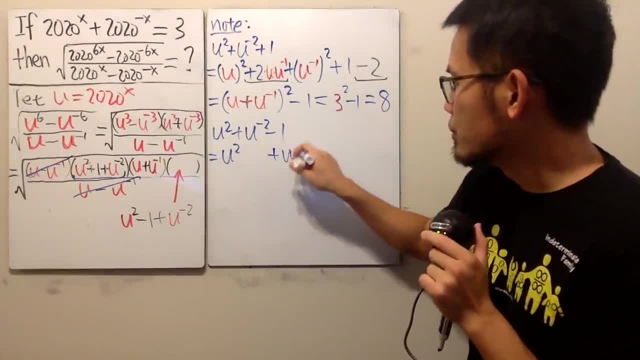 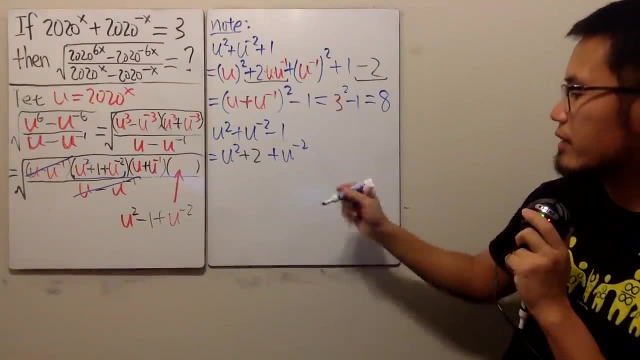 This: right here is u squared and then just leave a space plus u to the negative 2.. Right here, you know, we have to add the 2, just like this: In here we have the negative 1, but again, similar reason- we have to just minus 2, right here. 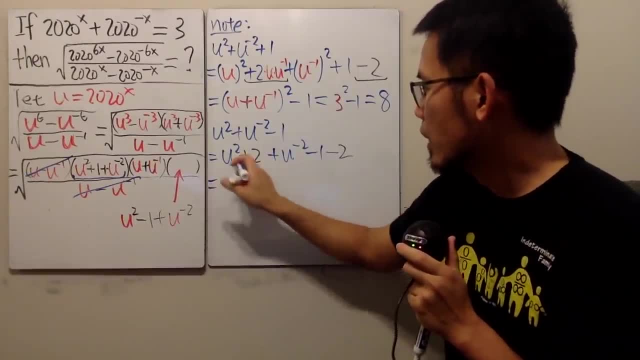 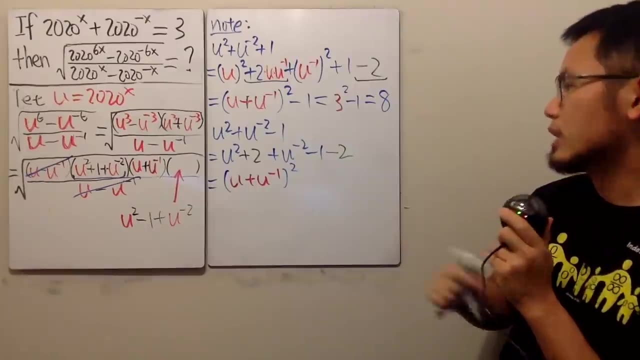 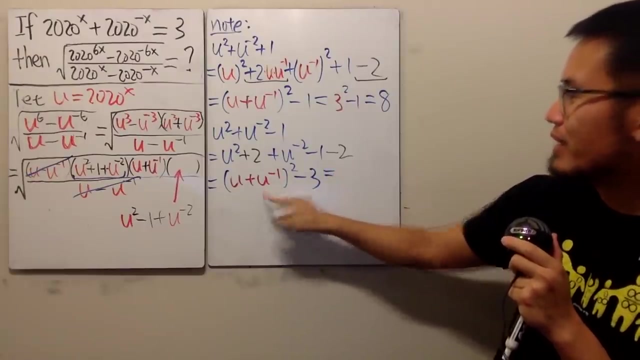 That's the idea. Well, here, all in all, we just end up with u plus u to the negative, 1, squared again, and this, and that will give us minus 3, which is very nice. All right, Put the 3 right here. 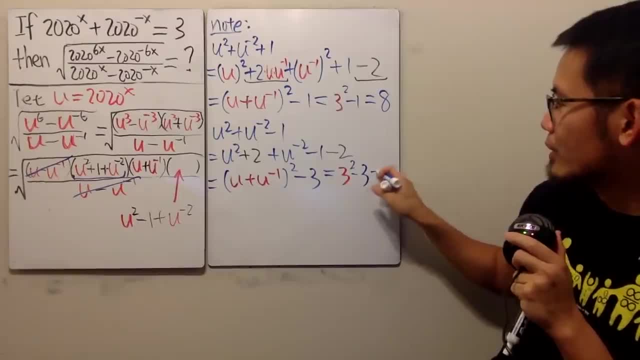 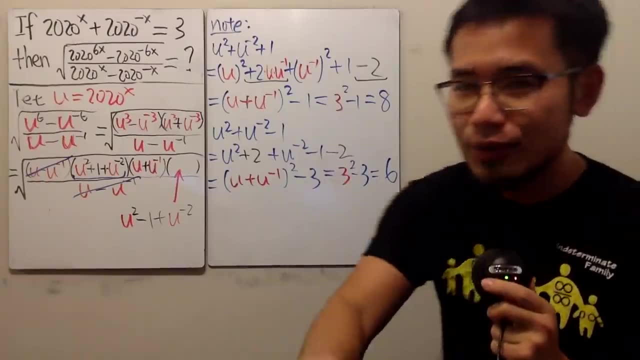 We have 3 squared minus another 3.. All in all, this right here is just going to give us to be 6.. Very good, huh? So that's pretty much it. We have all the stuff that we need First. this right here is 8, so I'll just put that down to be blue. 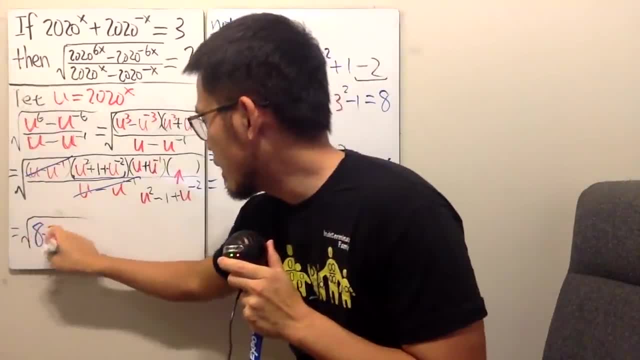 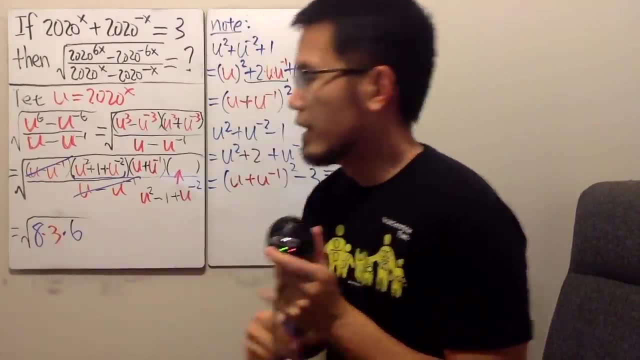 This right here is our 3, so we have 8 times 3 now. And lastly, this right here is the 6 that we have. so multiply by 6.. Well, 8 times 3 is 24.. 24 times 6 is 144.. 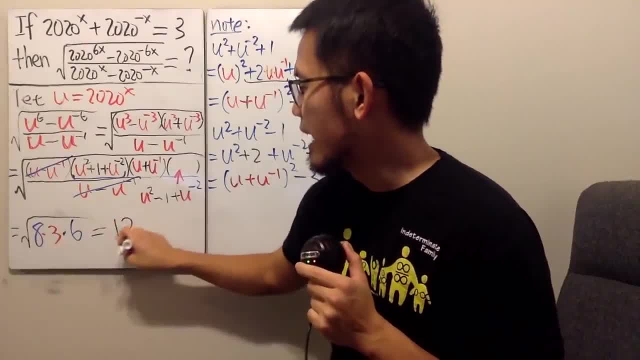 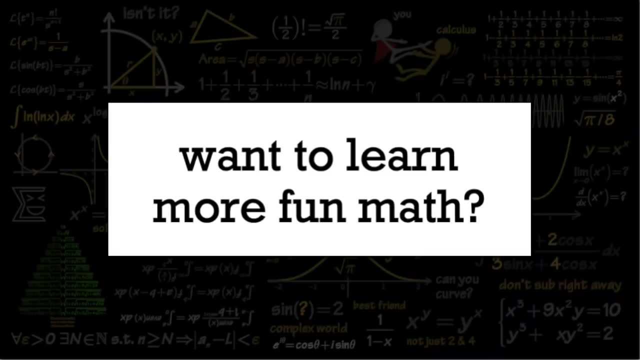 Altogether, take the square root. after that, We end up with a nice 12.. So the answer to this right here is equal to 12.. All right, If you enjoyed the question that we just did, then I think you'll also like Brilliant. 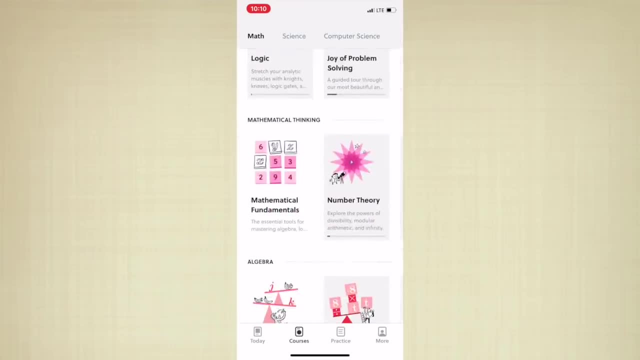 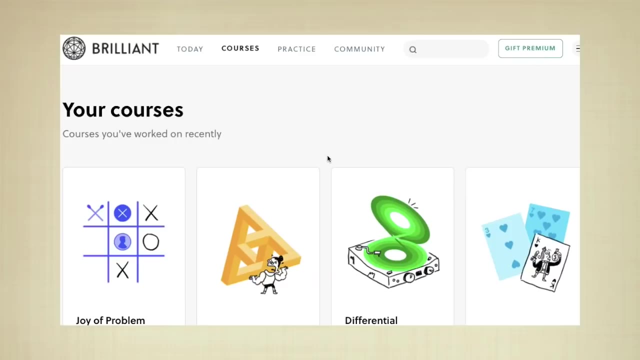 Brilliant is a problem-solving-based website and app with hands-on approach and over 60 interactive courses in math science and computer science, And you know many people are looking for online math resources right now, and whether you are a student trying to get ahead,